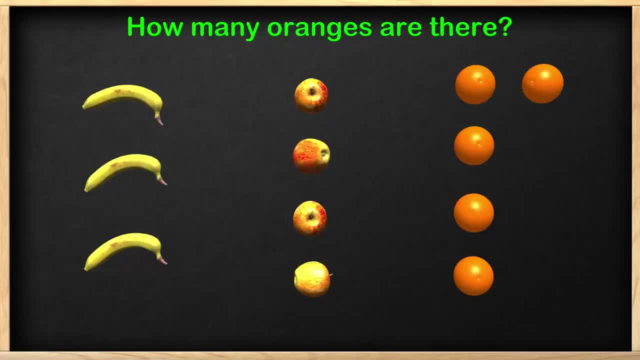 and apples are a distraction in this problem. Can you count how many oranges there are? We have five oranges. Great job, We organized our items and did not get distracted by the apples and bananas. that did not help us solve the problem. Let's take a look at another. 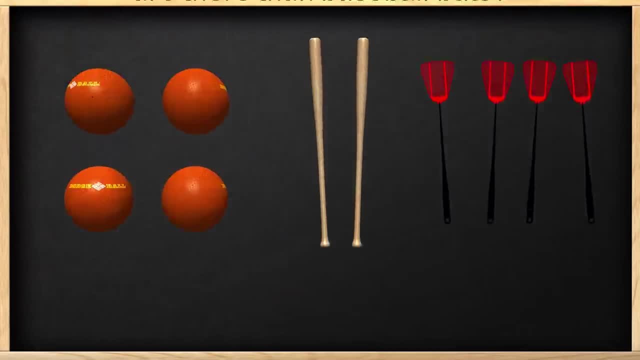 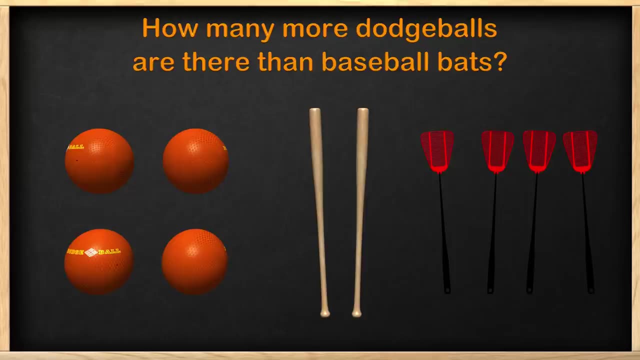 problem. The question asks: how many more dodgeballs are there than baseball bats? This question has three categories or groups. We have dodgeballs, baseball bats and fly swatters. Which group of objects do we not need to worry about in this problem? 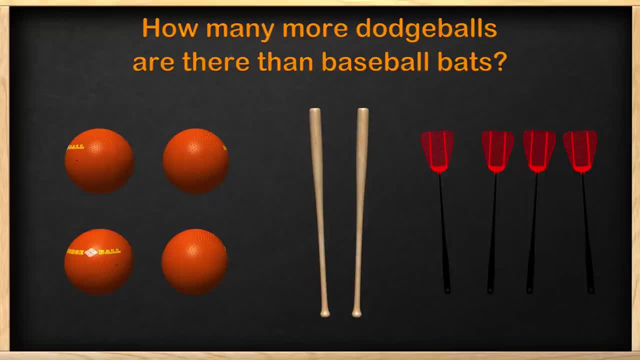 The fly swatters. Even though fly swatters are handy when pesky robot wasps come, they are not useful in this problem and are just a distraction. Let's move them to the side. We need to find out how many more dodgeballs than baseball bats To do this. we can pair. 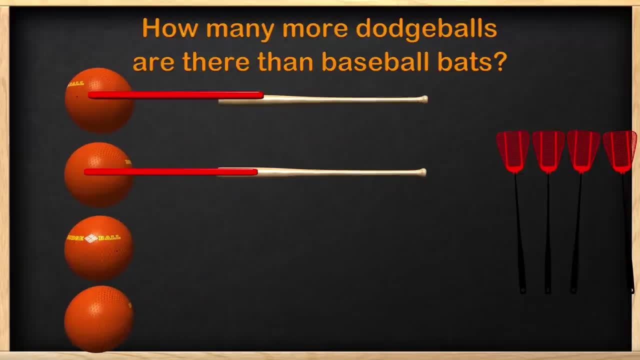 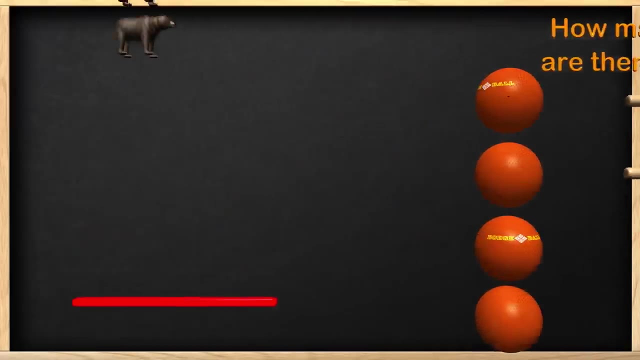 these objects together. How many dodgeballs are there that are not paired together? We have two. The answer is two. Awesome job, guys. Let's try one more and see if you can tell me if there is a distraction in the next problem. 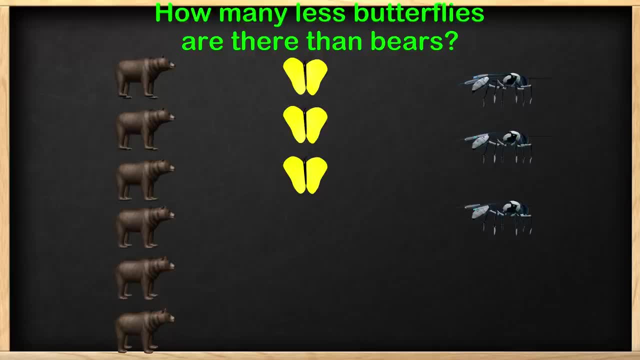 The question asks: how many less butterflies are there than bears? Now that we have the problem, can you tell me if there is anything here that is not needed to solve the problem? We don't need the robot wasps to solve this problem. Great job, Now to solve the problem. 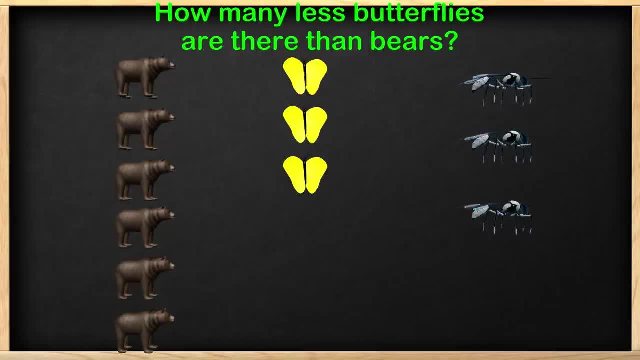 we can match up the objects like we did in the last problem. We match them up and we notice there are three more bears than butterflies. but that also answers the question: how many less butterflies? We have three less butterflies than bears. There are six bears and only three butterflies. We did it Awesome job. 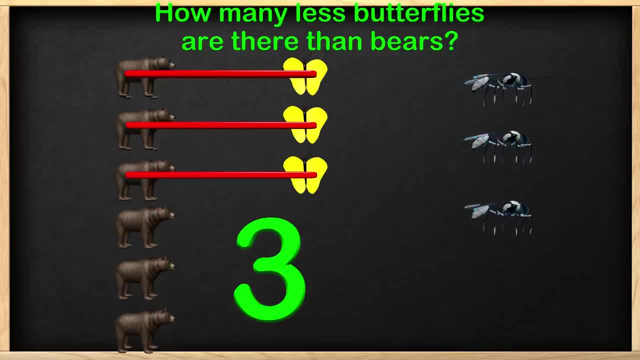 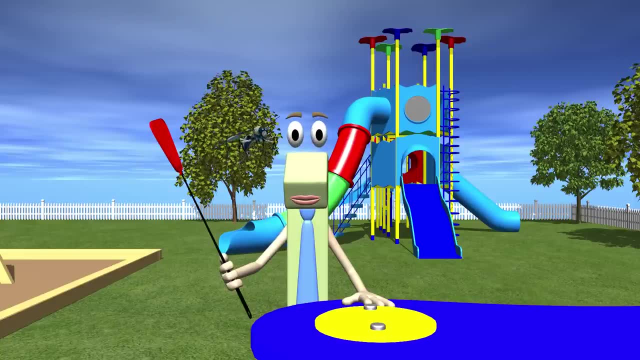 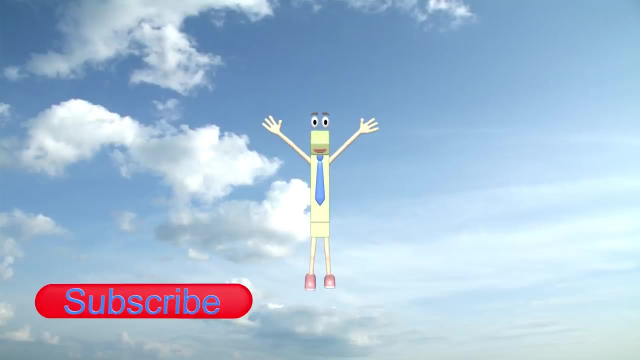 That pesky robot wasp is back again. I have a fly swatter, so watch out. Ouch, You have a few options here. You can click the video on my right or on my left to watch more awesome stuff. If you want to subscribe, click the big red subscribe button below. 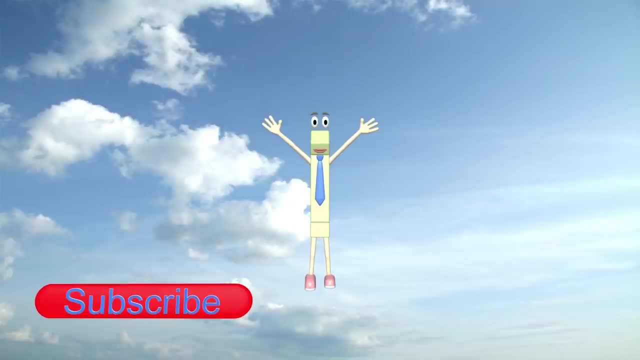 You might want to hurry and choose, though, because I can't hold on forever. Hurry, Choose, Uh oh. 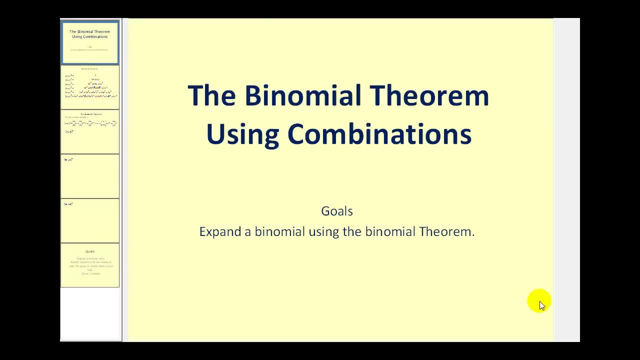 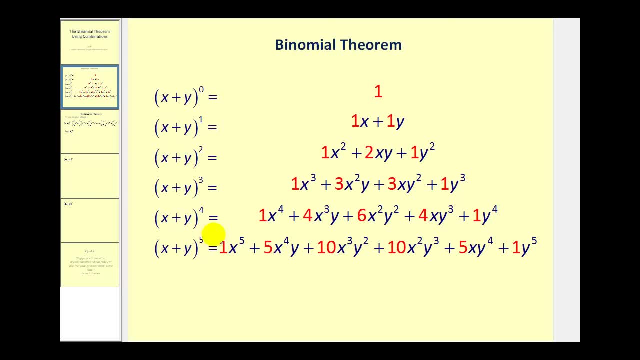 Welcome to a video on the binomial theorem. This video uses combinations to determine the missing factor rather than Pascal's triangle. Let's first take a look at the patterns we can recognize when we expand the binomial x plus y. For example, if we take a look at the quantity x plus y raised to the third notice, the 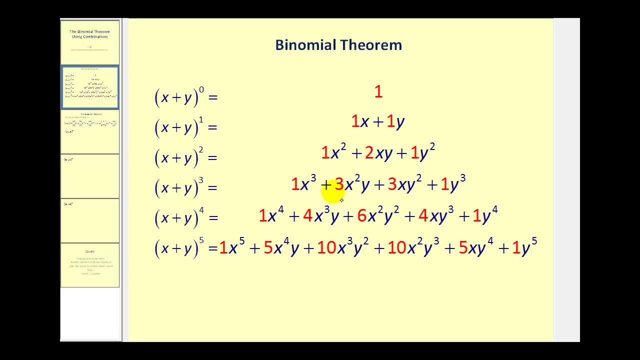 variable part of the first term is x to the third and the next term has x to the second. So the exponent has decreased by one. but then we start picking up factors of y. This would be y to the first. Notice: the sum of the exponents is still. 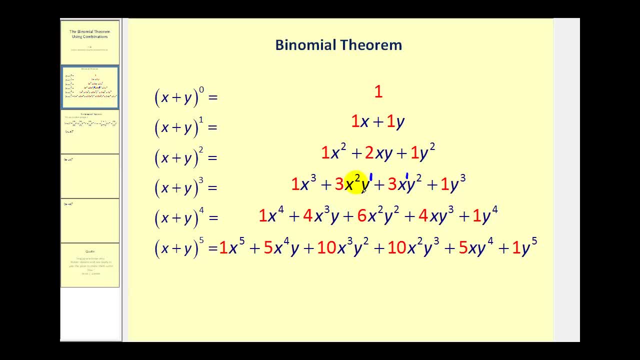 three, The third term, we have x to the first. so the factors of x has dropped by one again and we've picked up another factor of y all the way to y to the third. So if we jump down to the quantity x plus y to the fifth notice, we have x. 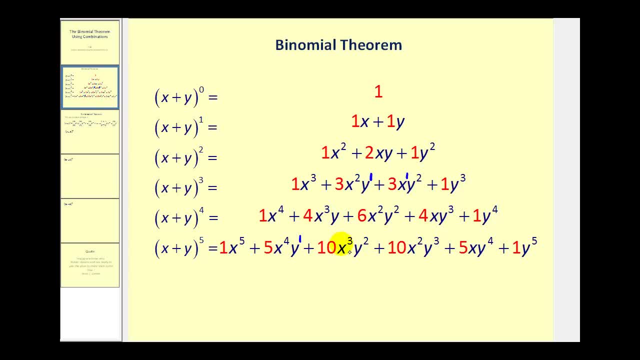 to the fifth, then x to the fourth, y to the first, x to the third, y to the second, and so on. So as we go from left to right, we lose factors of x's and pick up factors of y. Next in red we have these coefficients that we found last time. 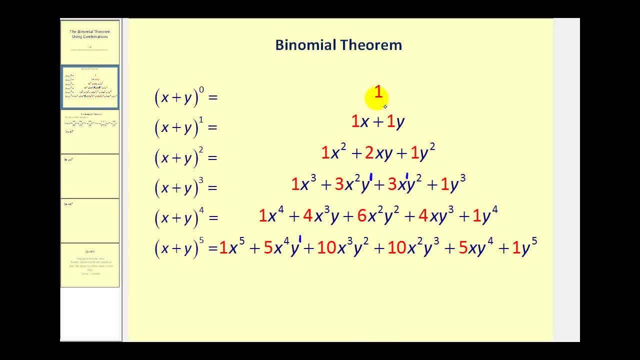 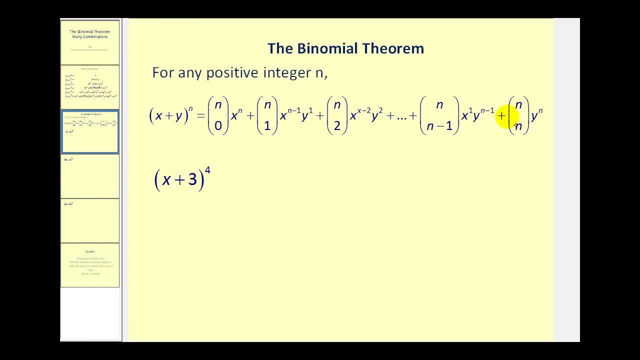 using Pascal's triangle, but now we'll take a look at how we can find them using combinations. Let's go and take a look at the binomial theorem. So this can look a little intimidating, but again, the idea here is to recognize the pattern. 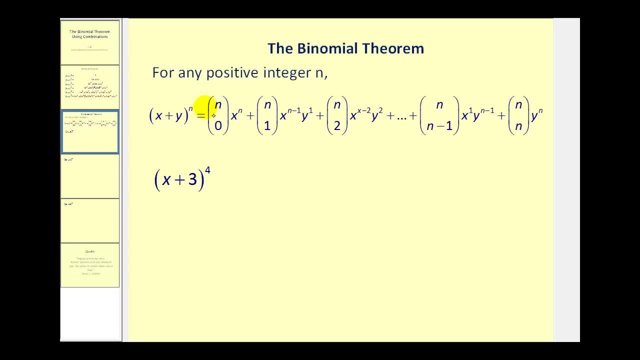 Notice: the exponent on x in the first term matches the original exponent. and then we decrease the factors of x by one and start picking up factors of y, And then those red coefficients on the previous screen can be found from these combinations: n choose zero, n choose one, n choose two all the way to n choose n.